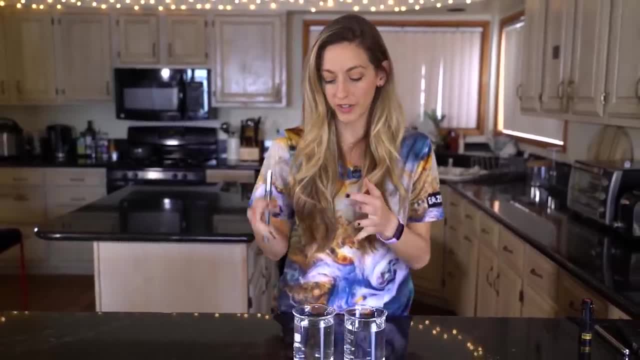 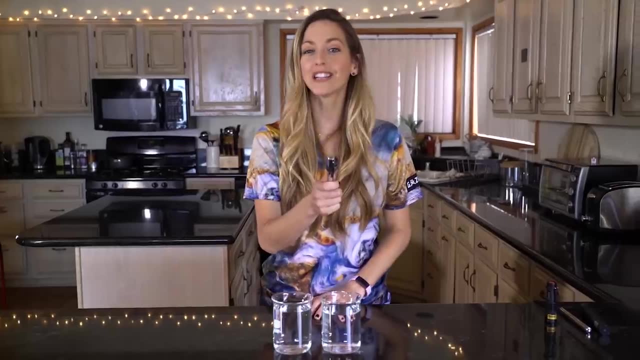 to shine the line through the water. What it's doing is scattering off of some of the water molecules or other impurities in the water, But the mystery liquid is very different. Can you guess what the mystery liquid is Before I tell you a quiz? And now is the. 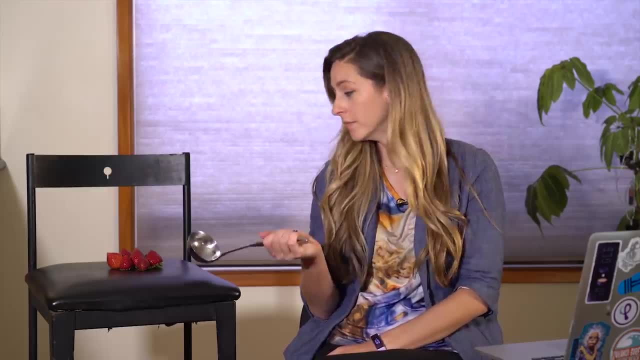 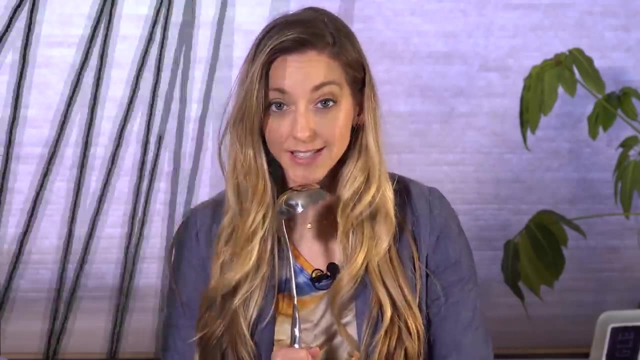 time of the show where I quiz fruit in my kitchen. Are you ready? Well, let's jam. Here's the question. Since the laser was invented in 1960, what is the coolest use for lasers? Is it measuring the distance to the moon? Laser tag Detecting gravitational waves? 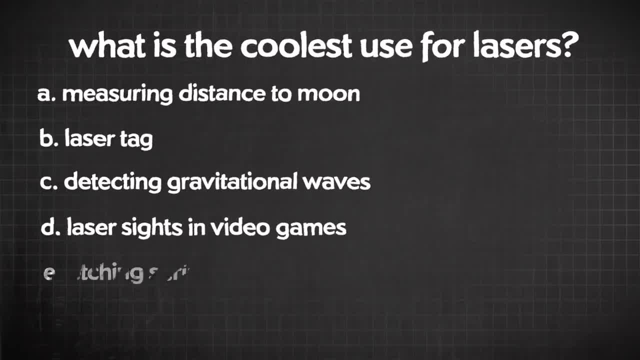 To give gamers a reality-based sense of what they're doing. Is it measuring the distance to the moon And, if so, what is the best reality-based way to sight their targets in video games? Etching itty-bitty serial numbers onto diamonds To control and cool individual. 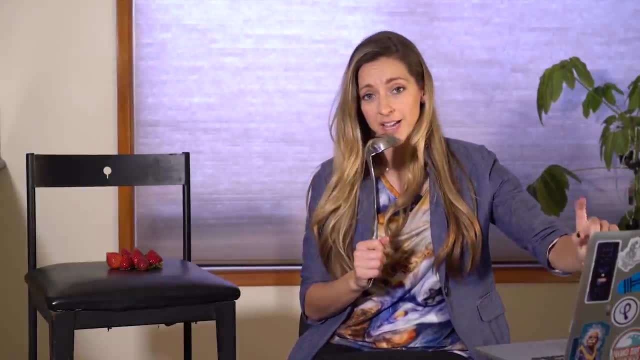 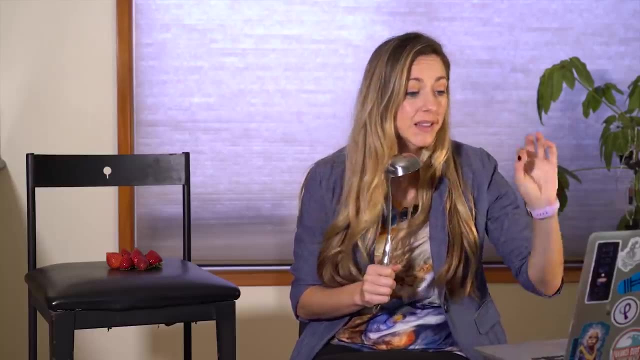 atoms. And the answer is: Ah, yes, laser tag was a close second, You were very close- But the answer is actually F to cool and control individual atoms. Laser cooling is literally the coolest use for lasers and it's a real and crazy thing- We can use lasers. 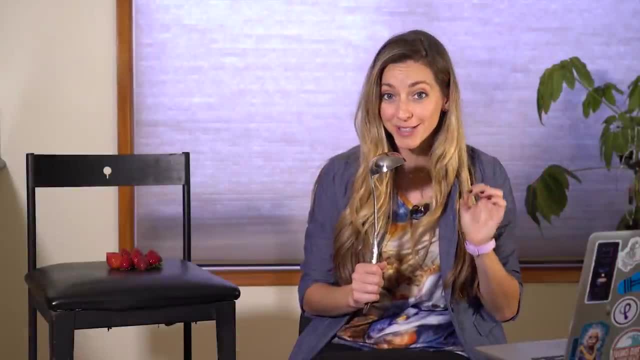 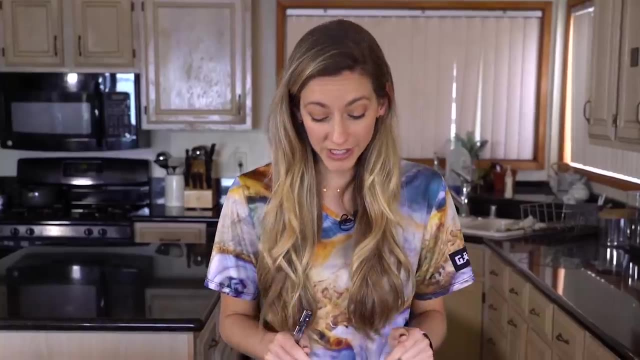 to cool individual atoms and molecules down to near absolute zero. OK, back to you, Diana. Thanks, Diana, Mystery liquid. It's actually tonic water. Tonic water contains an ingredient called quinine, And when you shine the violet light on the tonic water, 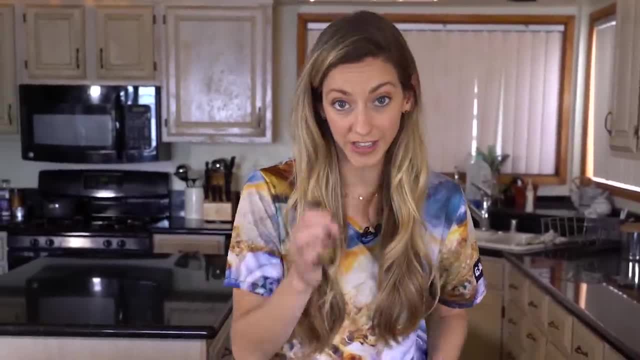 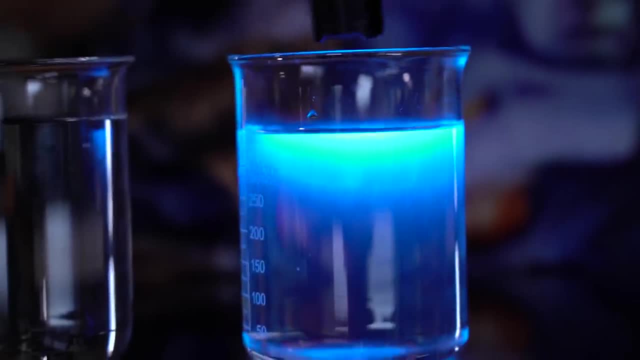 it glows, It fluoresces. Check what happens when I shine an ultraviolet light First on the water and then on the tonic water. Yeah, So fluorescing is this process where higher energy light like ultraviolet or violet light, is absorbed. 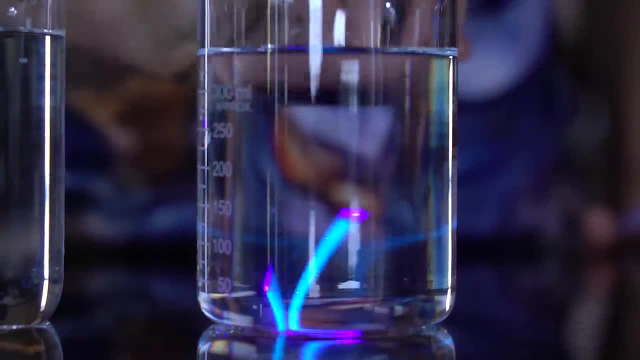 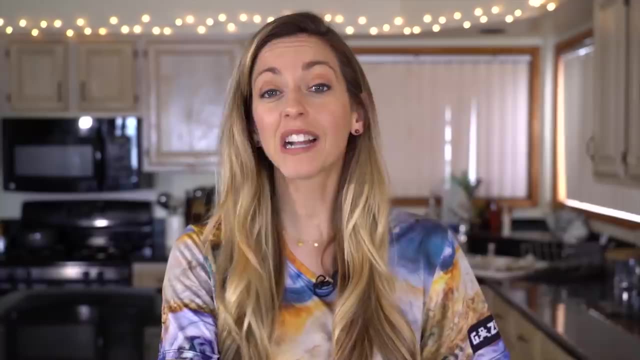 and then lower energy light is emitted. It glows lower energy colored light. So in comes ultraviolet, out goes blue. That's what's happening with the quinine. But regular water is cool too. Here's a fact about water. 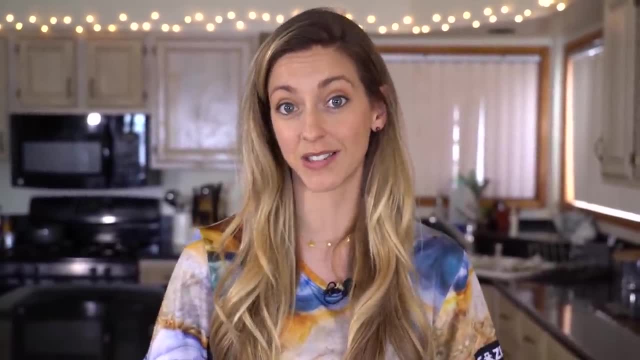 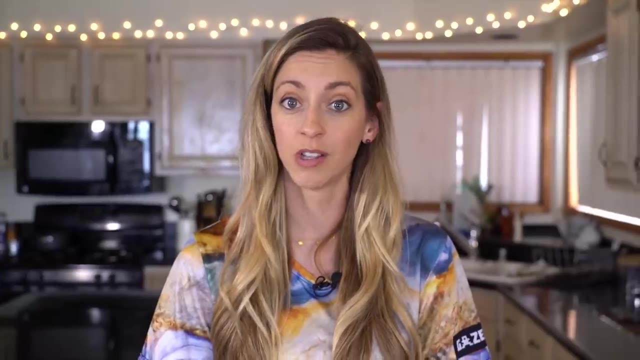 Of all the water on Earth, only 1% is used for human activities like agriculture, plumbing, drinking- which means that over your lifetime, you will most likely drink some water molecules that a dinosaur peed out. Cool, Next one. 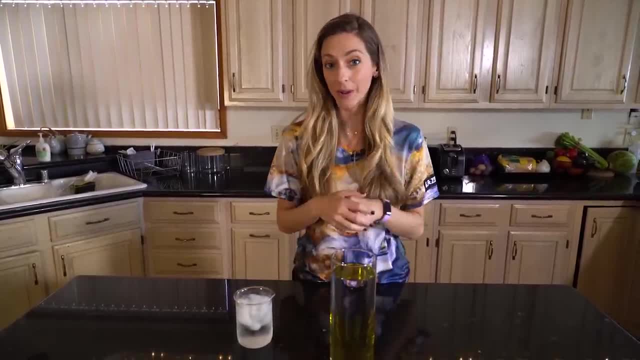 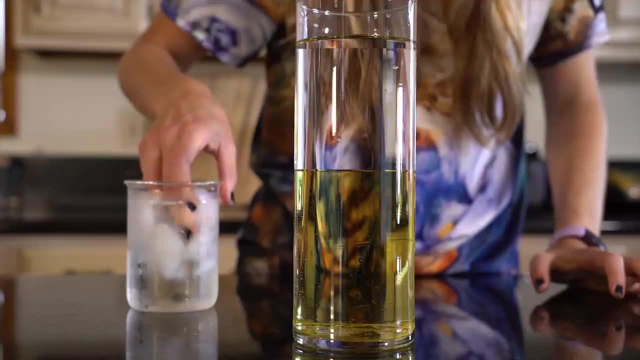 In this container. I have some oil And I'm going to drop an ice cube into the oil. Now my question is: is the ice cube going to sink float, explode or something else? Let's see. Why would the ice cube stop in the middle? 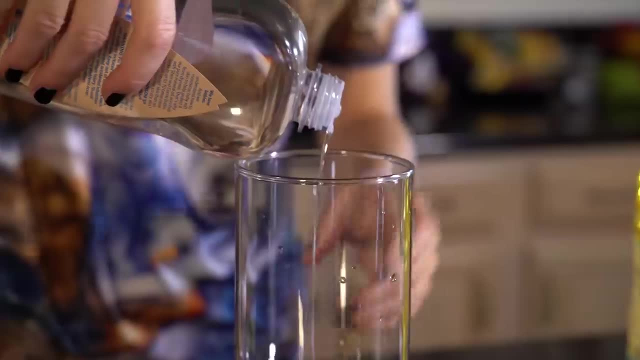 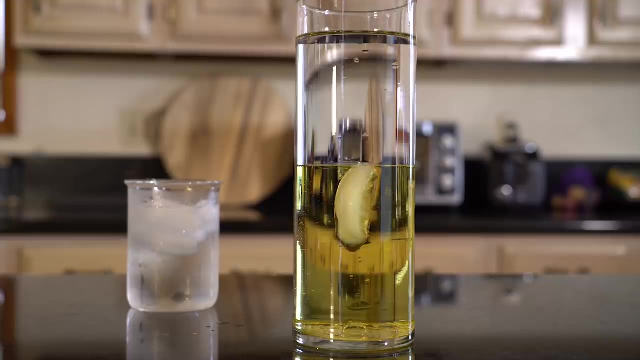 Well, this was a tricksy one. I actually poured two different types of oil in here. There's vegetable oil on the bottom and baby oil on the top, So the ice floats right in between, or maybe a little bit lower, into the vegetable oil. 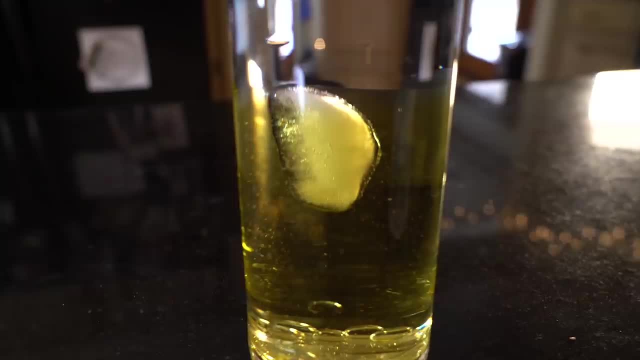 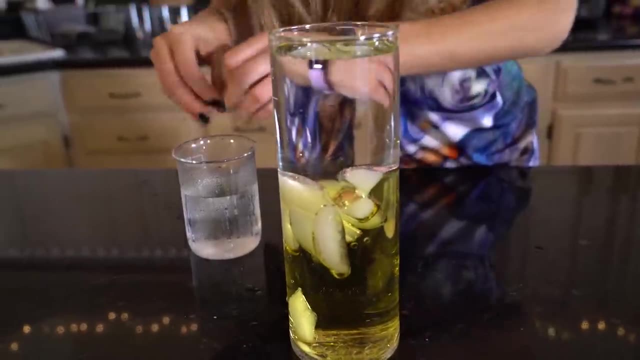 Now, when the water from the ice melts, it increases in density to nearly 1 gram per centimeter cubed, so the water sinks to the bottom of the oil. The water initially sticks to the cube, weighing it down, and then drips off and the cube bounces back up a little bit. 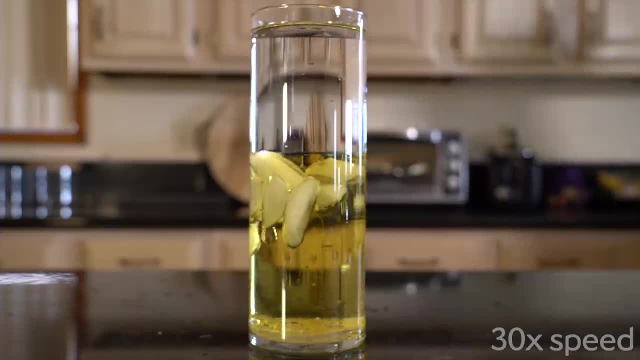 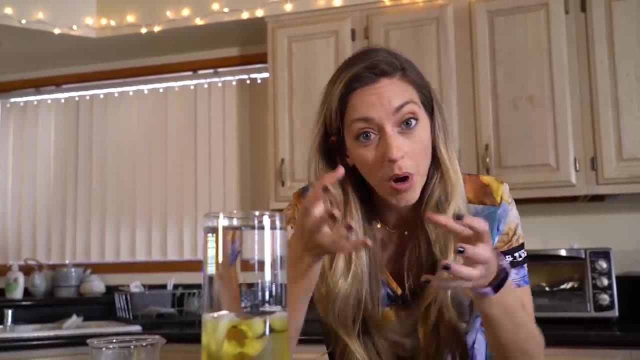 Now I have a question. If you were holding an ice cube in a boat and the water was dripping off your hand into the bottom of the boat, would the boat go up and down like these ice cubes as the water dripped off and splashed onto the floor? 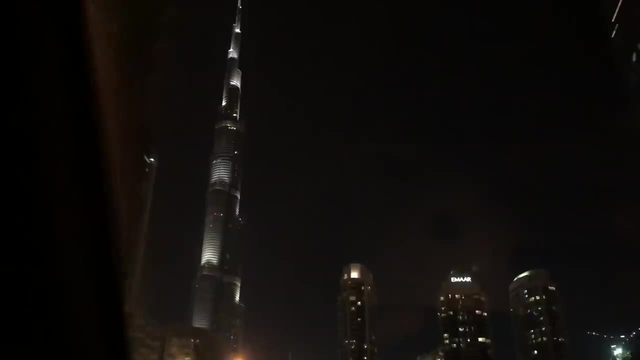 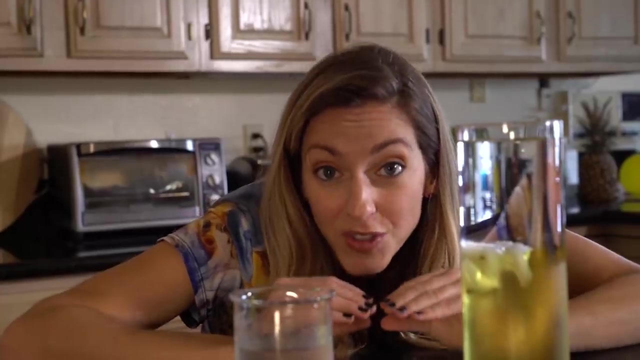 Leave your answer in the comments below. Here's a fun fact about density. If I wanted to fill the tallest building in the world, the Burj Khalifa, with water vapor- by boiling water- I would only have to fill 1 tenth of one story with water. 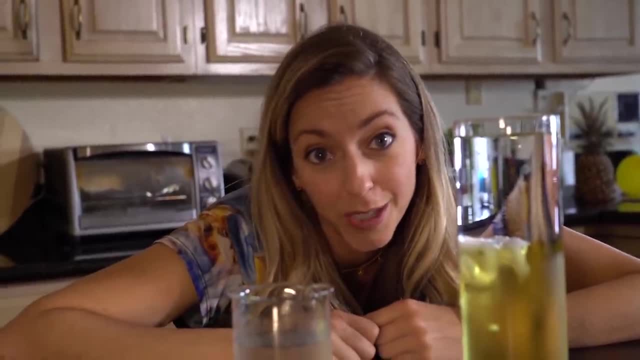 and boil that to fill the rest of the 163 stories, which I'm pretty sure are stories with water vapor. Although I'd have to fill the story, that's the average volume of the rest of the stories, but you get the idea. 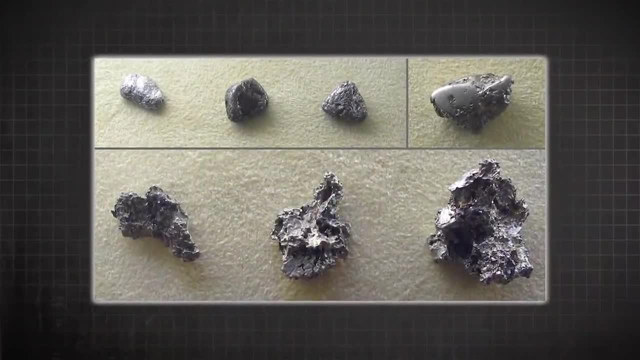 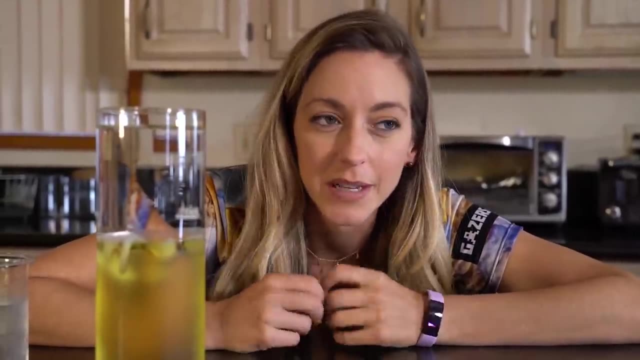 Another crazy cool fact about density: The densest material naturally found on Earth is a metal called osmium, and it has a density 22 times that of water. Now how does that compare to the lightest material, aerogel? It's a man-made material, but it's really light. 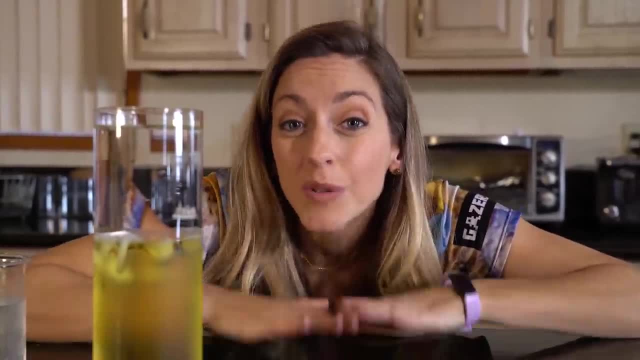 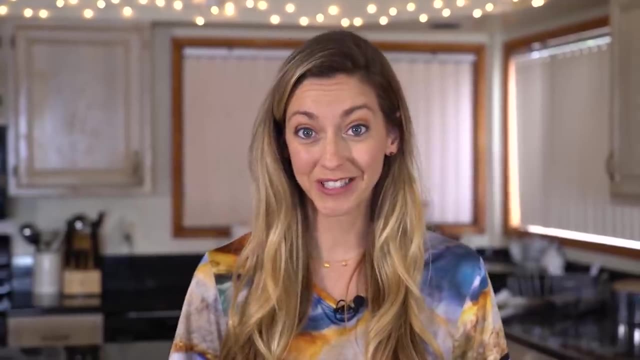 Now, if you had a sugar cube size of osmium, it would weigh the same as 20,000 sugar cube sizes of aerogel. That's crazy. All right, Next experiment. This one is really cool. This is actually one of the first experiments. 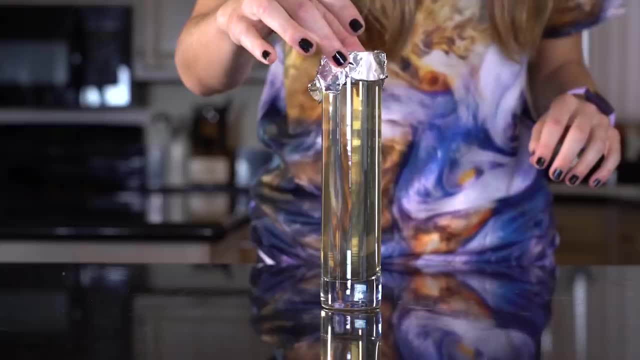 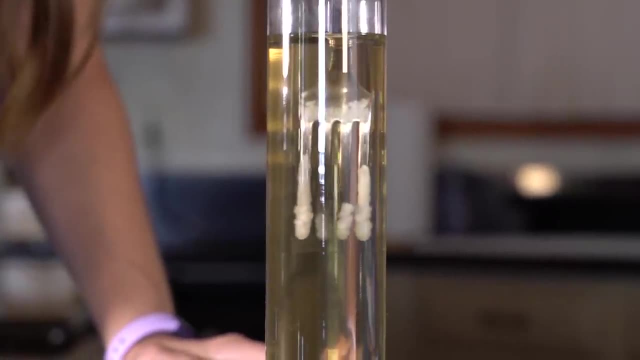 I remember ever doing in third grade, but we're going to do it bigger. Here's another mystery liquid. I scratched off a bit of residue from when I made the liquid and watch closely. A lot of people call this hot ice and in fact, 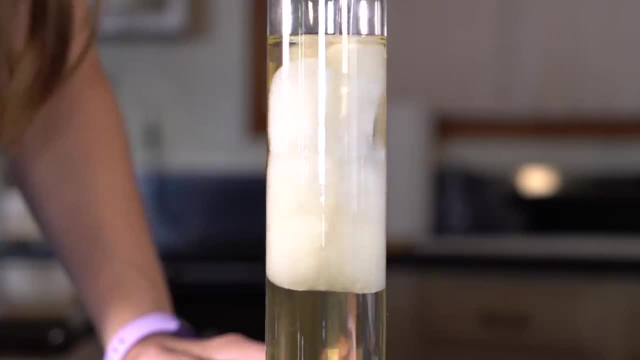 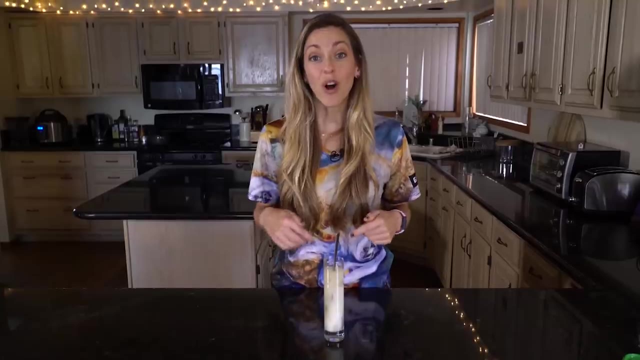 it is pretty warm to the touch. We measured the temperature before and after it crystallized, and it rose nearly 30 degrees Fahrenheit. So what do you think this liquid is? What is it? Well, it's called sodium acetate and you can actually make it with adult supervision. 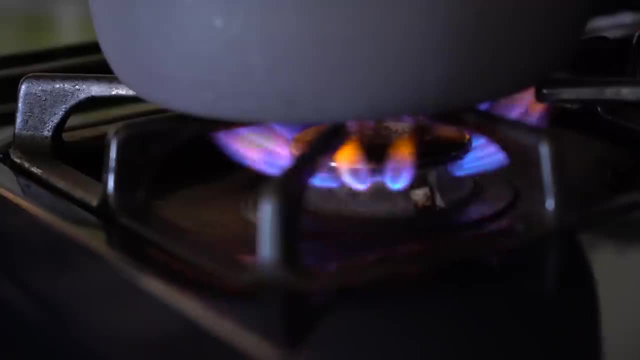 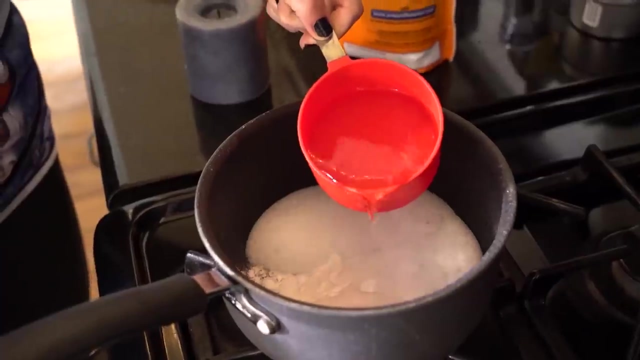 by mixing a quarter cup of baking soda with a liter of vinegar, which we all know makes CO2 gas which you can actually scoop out and pour out candles with. That's a bonus experiment, But the other stuff you make is sodium acetate. 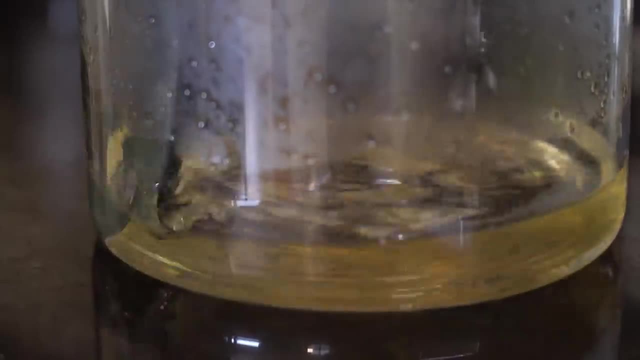 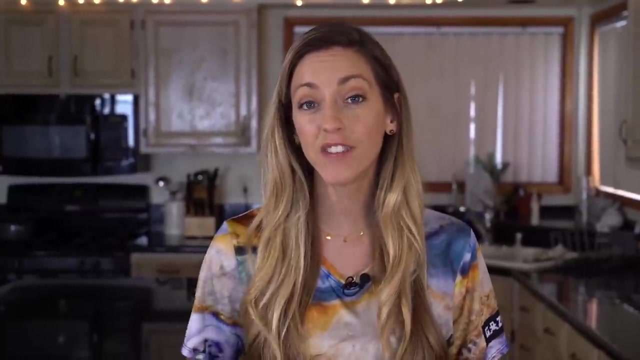 Then you boil that stuff for about an hour and then pour it into a jar and you can just set that aside, cover it on the table or refrigerate it until it's relatively cool to the touch. But sodium acetate freezes at 58 degrees Celsius. 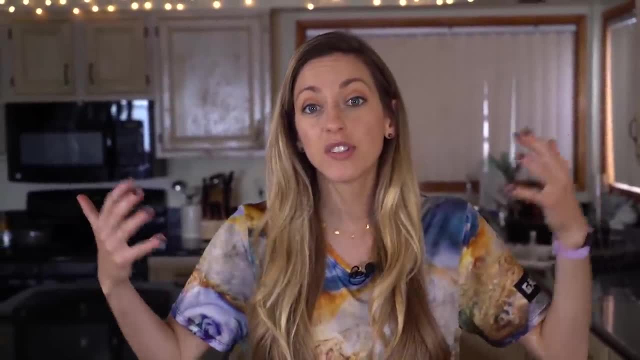 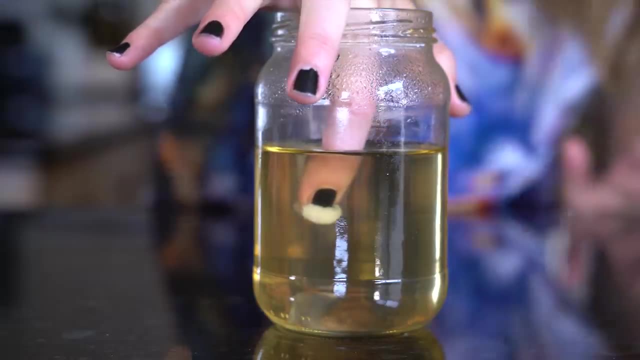 So what you did when you put it in the refrigerator and let it cool down, is you actually super cooled it. You can super cool water bottles. You can put the water below the point where it would solidify into ice, But the thing is it needs a nucleation site, a place. 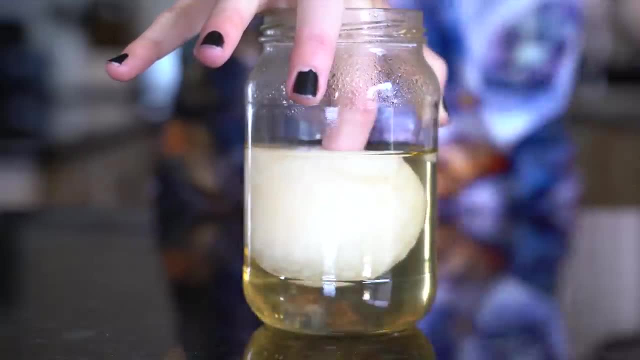 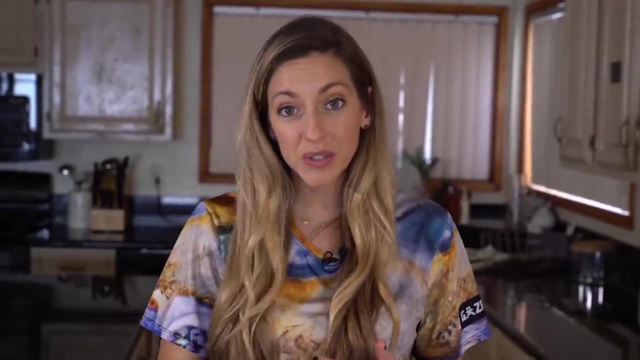 for the ice crystals to start growing, So you can only do that with really pure water. But sodium acetate is really stable stuff so you can super cool it easily And then you need to put some crystals like the residue we used, or introduce your finger. 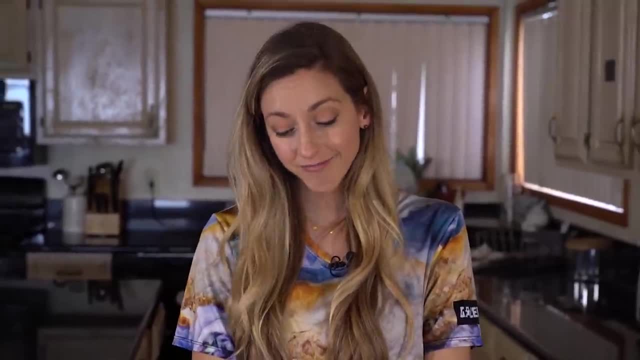 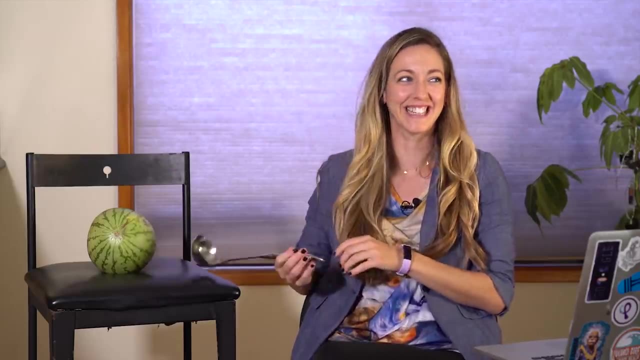 or shake it around or something like that in order to get it to start crystallizing, And that's hot ice Diane. I'm so sorry to interrupt with this segment. We have an exclusive interview with this melon. Two of these facts are true and one is a lie. Can you guess which? Here are the facts. Sodium acetate is used to clean out drains because it dissolves hair tissues. Sodium acetate is used in portable hand warmers. Sodium acetate is used to flavor salt and vinegar potato chips. And the answer is: do you need a life? 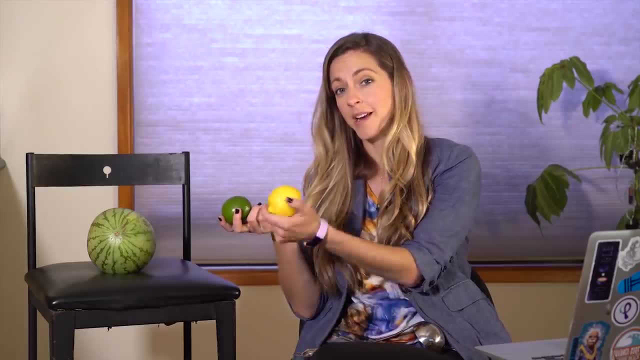 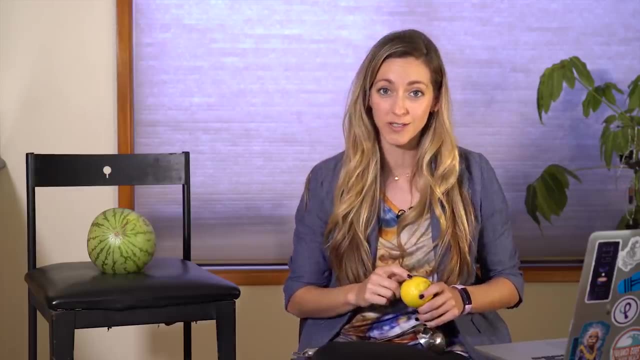 lime. some help from some other citrus, perhaps some lemonade? Ah, that is correct. The first one is a lie. Sodium acetate is used to flavor food and it is used in hand warmers, But it's sulfuric acid that is used in drain cleaner. 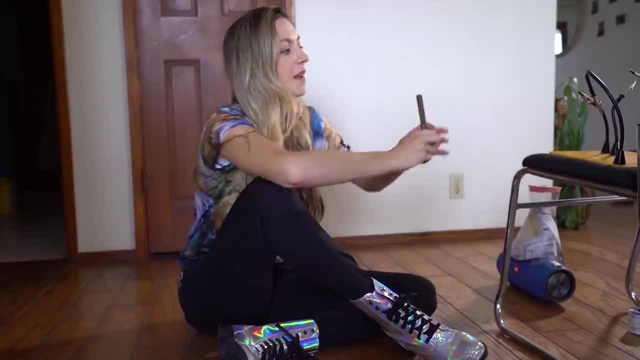 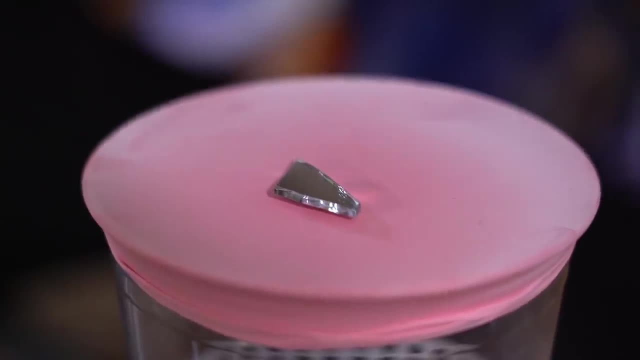 All right, Back to you, Diana, For the final experiment. I have a laser And I'm going to put it on this little contraption here to hold it steady. The laser's pointing down at a piece of mirror, The mirror's on top of a balloon stretched over a cup. 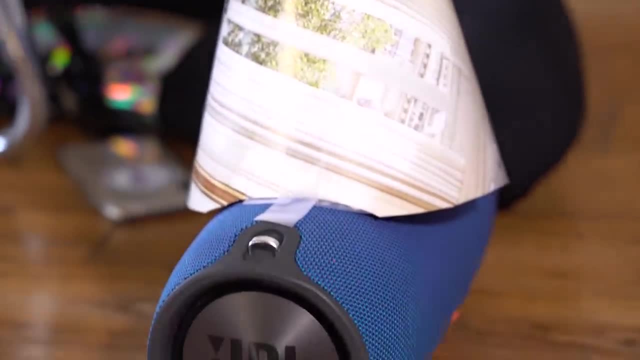 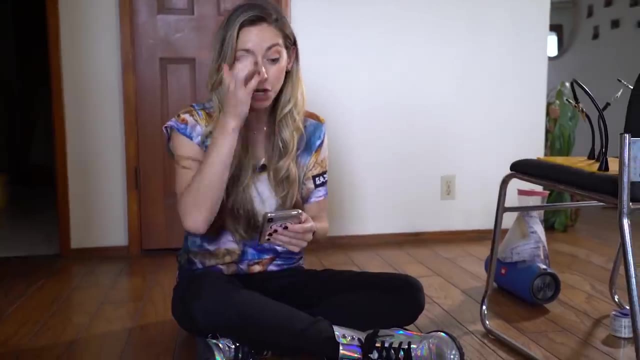 with the bottom cut out And the cup is taped to a cone. I made out of some thick paper That all is taped to a speaker And out of the speaker. I'm playing a single tone, a single note. So I have this app called Sonic. And I'm just picking a frequency like 65 hertz. This is what 65 hertz sounds like. I can go up in frequency, which means the pitch goes up. Here we go, 75,, 85. Now, when I turn the laser on and the laser 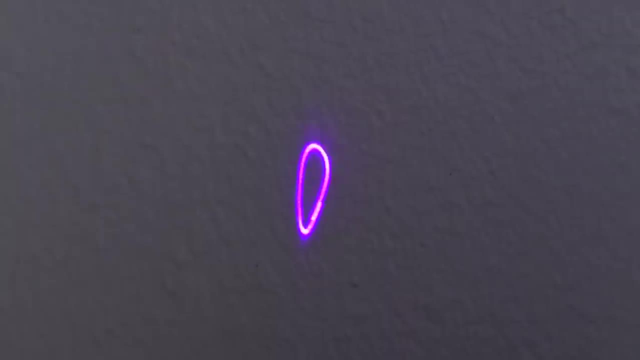 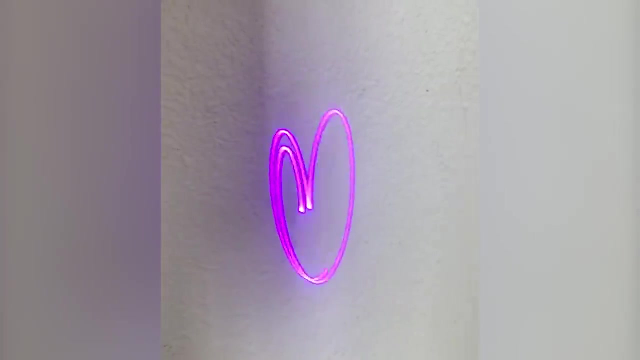 reflects off of the piece of mirror. check out what happens on the wall. Now, if I add another frequency, you get even more complex motion. What we're seeing looks like an animation. It's crazy. Even in real life it doesn't look like this could be real. 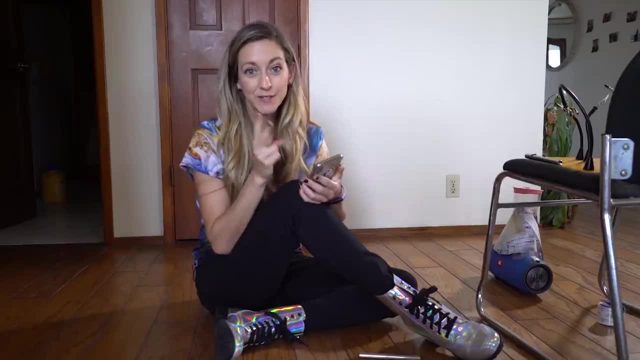 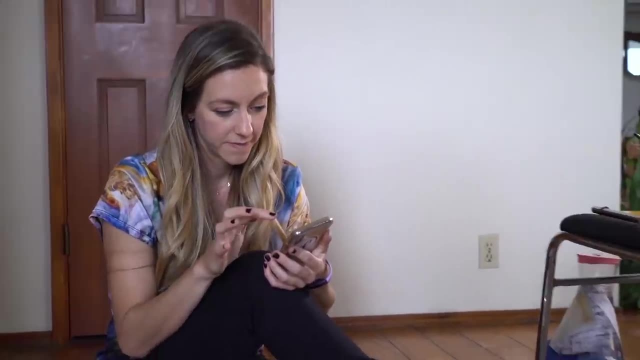 So this app, Sonic, only does one frequency, but I figured a way to do two frequencies by getting a second app called Function Generator And I played them both at the same time. This is what that would sound like. This is 85 hertz plus 110..